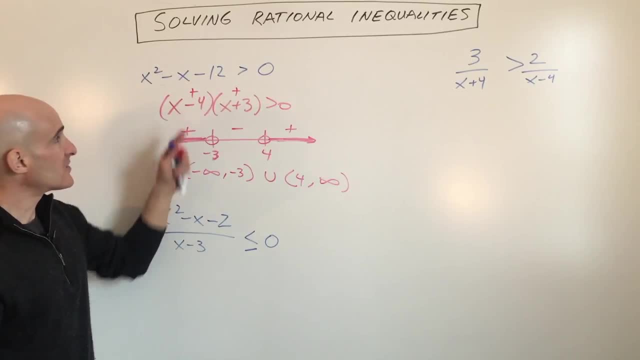 regions would make this inequality true. Okay, so that's just a regular inequality. Now we're going to talk about the rational inequalities And this example. here, the first thing I'd recommend you do is just factor it and then we'll set the factors to 0. So if we do that, we get x minus 2, x plus 1,. 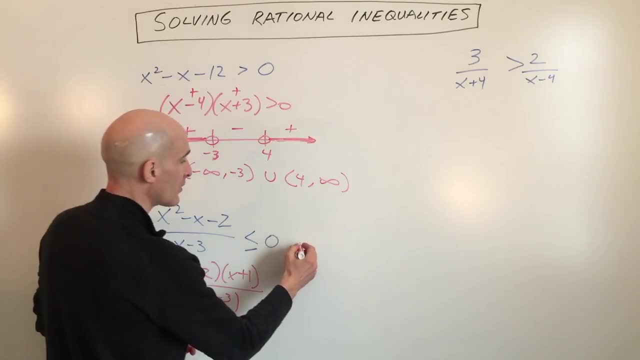 x minus 3. okay, we're going to go to the number line and we're going to plot these, set these factors to zero and plot those points. so we get: x is 3, okay, so I'll just put 3 here. we get 2, so I'll put 2 there and negative 1, because I put them in order from lowest to highest. 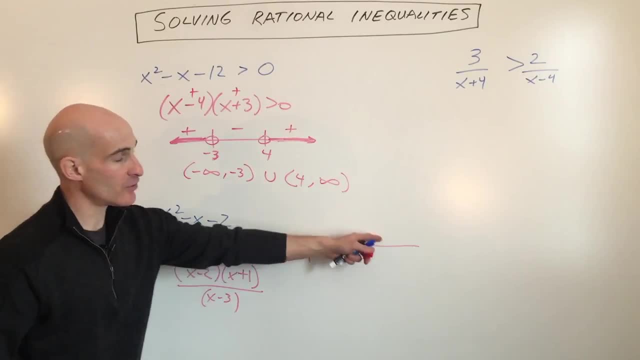 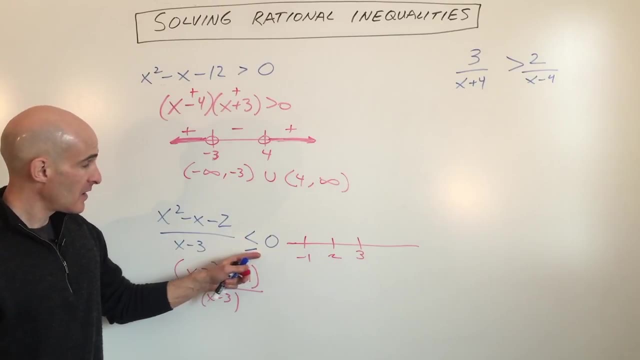 and then what you want to do is you want to pick a point in each of these intervals and test to see if it's positive or negative. before we do that, we're looking for where this is less than or equal to 0. now, if the numerator is 0 and the denominator is not simultaneously 0, then this is. 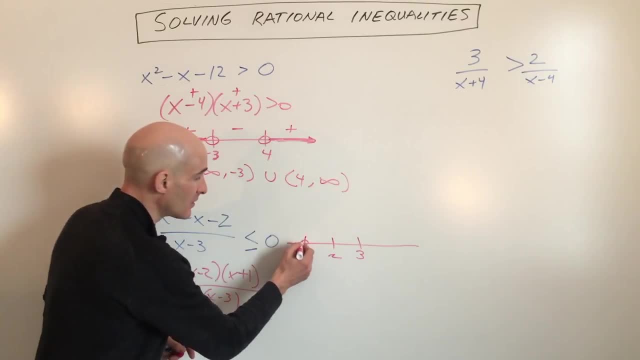 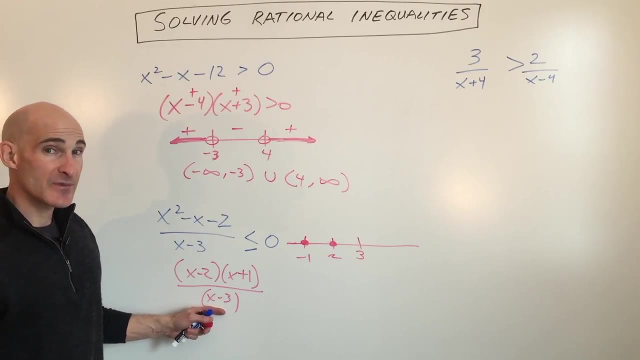 going to be equal to 0. so at 2 and negative 1, that's going to make the expression okay, equal to 0. but the denominator we know cannot be 0, because you can't divide by 0. so over here at x, equals 3, even though this is less than or equal to 0. we can't divide by 0. this is going to be an. 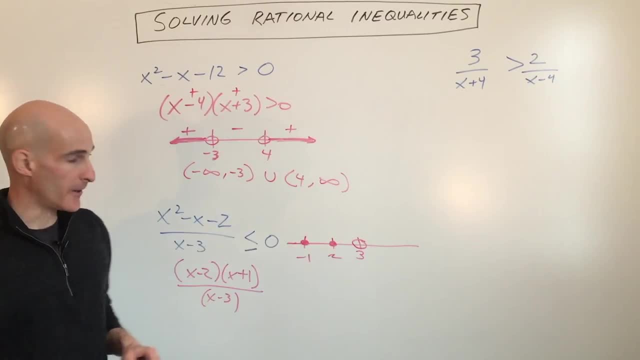 open okay circle. it doesn't include that point. now we're going to test our intervals, so let's see if we can put in negative 2. so we put in negative 2, we're going to get a negative times a negative and that would also be negative. so a 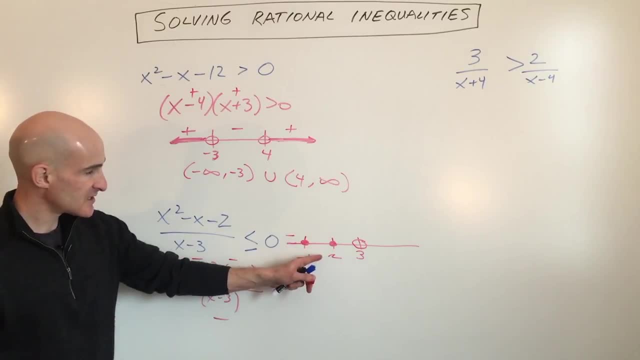 positive divided by a negative is a negative. if we do, let's say 0 is always a good one, that's going to be negative times a positive divided by a negative. so that's a negative divided by a negative, which is positive. so we're just doing a sign analysis. we're not so concerned with the 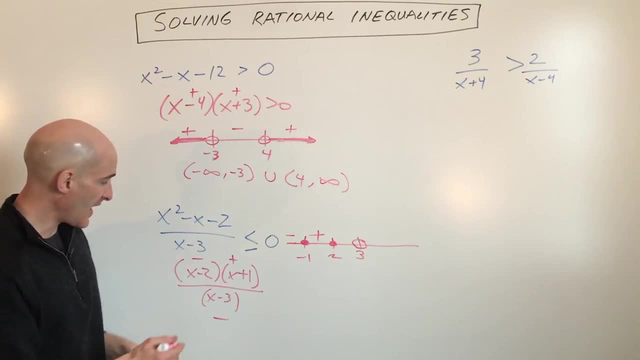 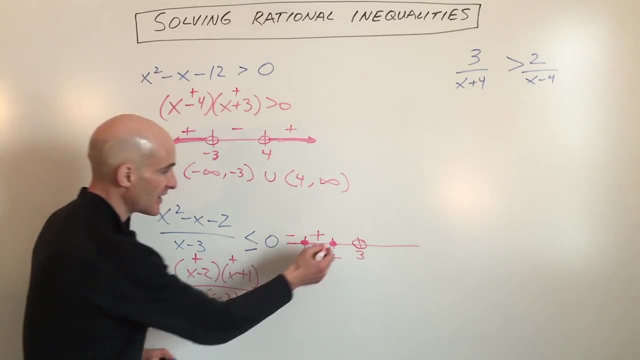 number, just whether it's positive or negative. and if we pick 2.5, we're going to get positive, positive and negative. so two positives multiply to a positive. divided by a negative is a negative, and if we pick four, we get positive, positive, positive. so that's going to be. 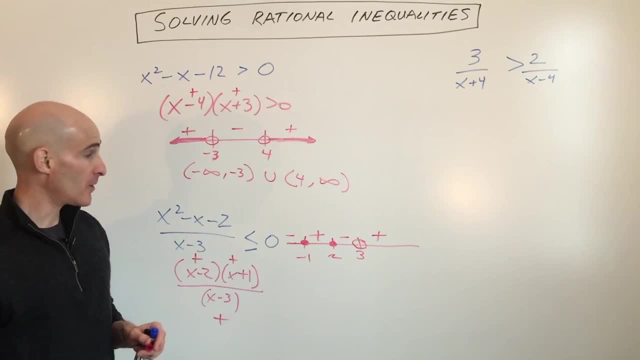 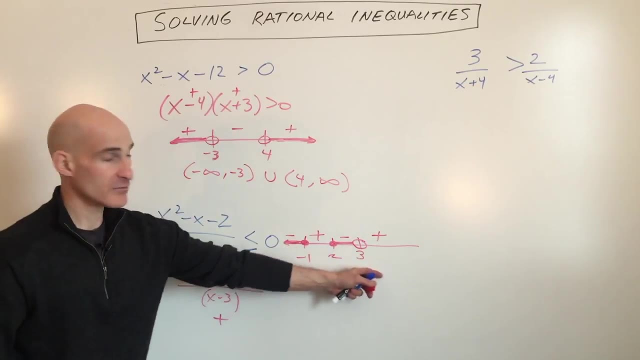 positive. now we're interested in where it's less than or equal to 0. so it's just going to be in this region here and this region here, and so again, if we think about going from low to high, or negative infinity to positive infinity, this is going to be negative infinity to 1. I'm using a. 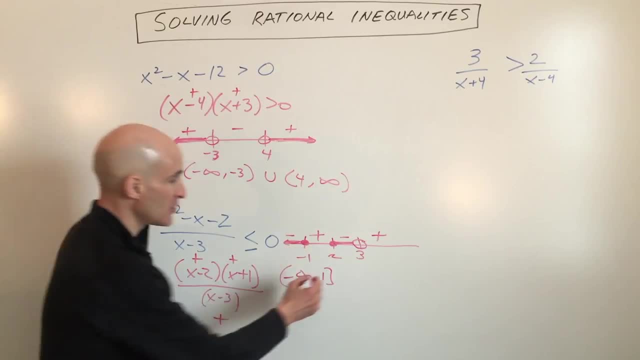 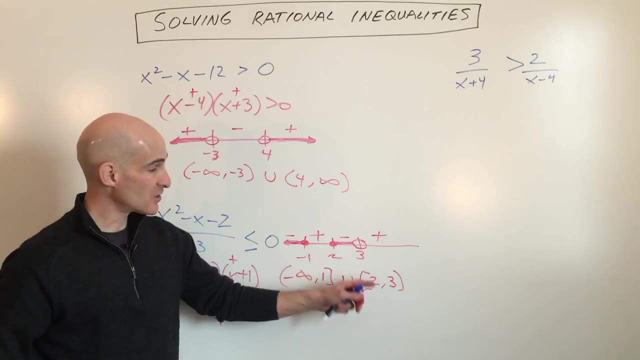 square bracket because it includes 1. okay, union 2 to 3: it includes 2, doesn't include 3, so I use a parenthesis: okay, this is curved for 3, square bracket for 2 because it includes 2, and so if you're in these two regions, that's going to be, this expression is going to be less than or equal to 0. 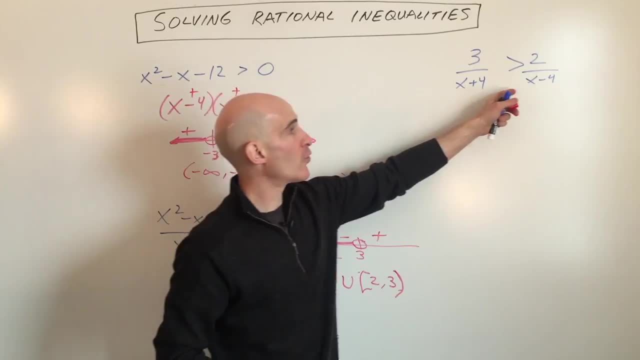 okay, the last one a little bit trickier. what we want to do is want to get everything on one side of the inequality, set it to 0, and then we're going to get the other side of the inequality set it to 0, and then we're going to get the other side of the inequality set it to 0, and then we're going to. 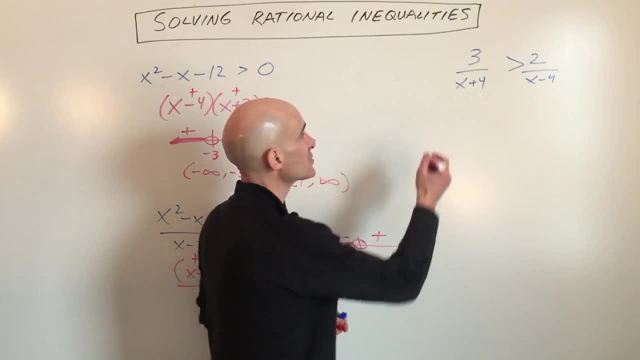 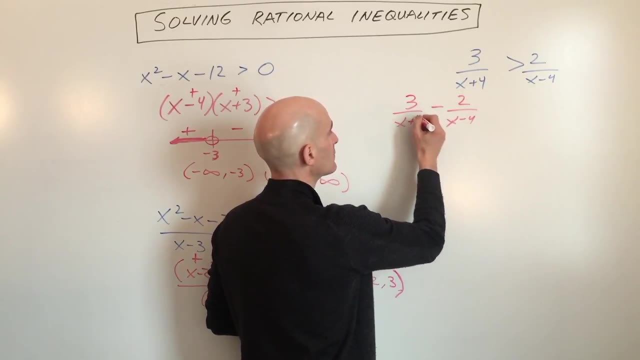 0. okay, and proceed from there. so let's do that. so I'm going to. first thing I'm going to do is I'm going to subtract minus 2 over x minus 4, get a common denominator which is just going to be x plus 4, x minus 4. here I'm going to multiply by x minus 4 over x minus 4, so that's going to give you. 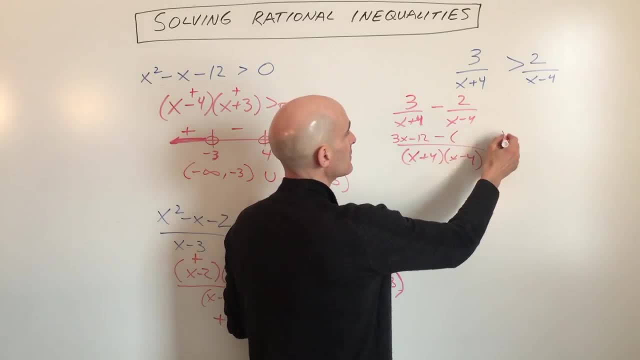 3x minus 12. minus this is missing an x plus 4. so I'm going to multiply the top and bottom by x plus 4, so that gives you 2x plus 8 and if we combine like terms we get 3x minus. 2x is 1x negative. 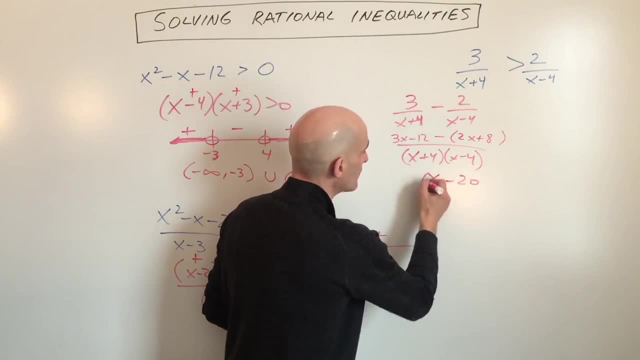 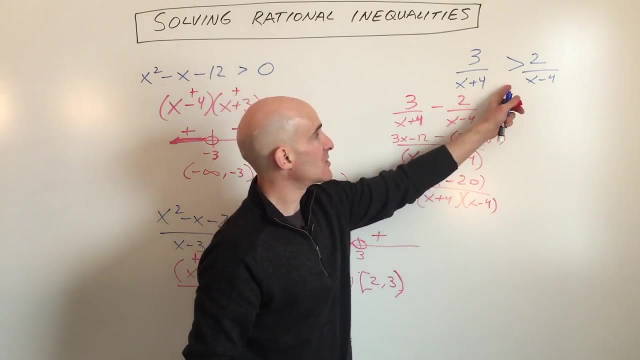 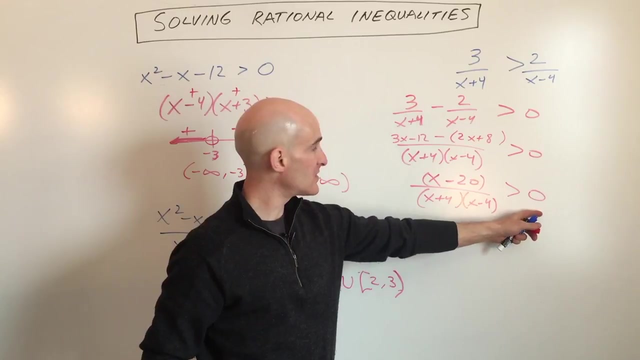 12 minus 8 is negative 20. okay. and then the denominator. we have x plus 4 times x minus 4. okay. now we're interested in where this is greater than 0. we got everything on one side, want to set it to 0, so greater than 0, so we're going to do the same thing we did in the other. 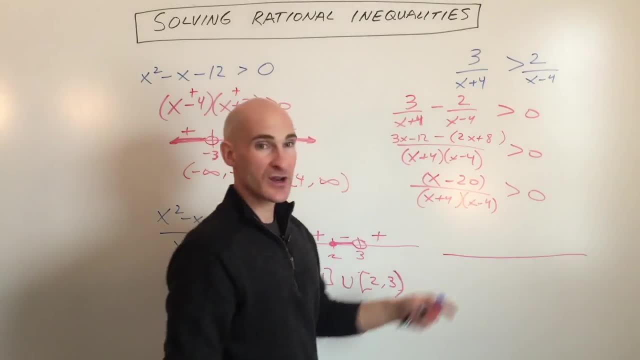 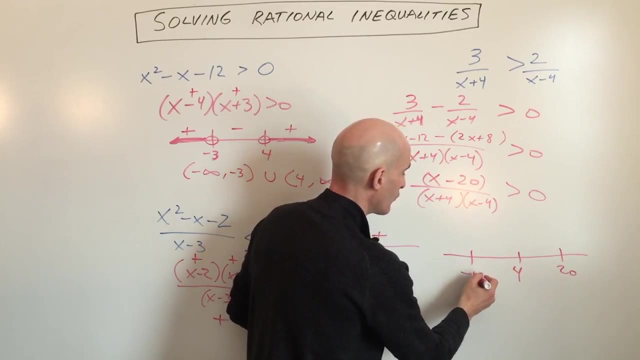 problems. we're going to set all the factors to zero, numerator and denominator. so we have 20, we have 4 and we have negative 4. now negative 4 and positive 4. okay, it cannot equal 0, so these are going to be open circles.